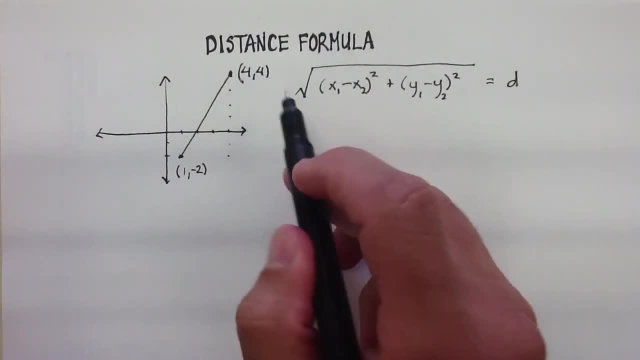 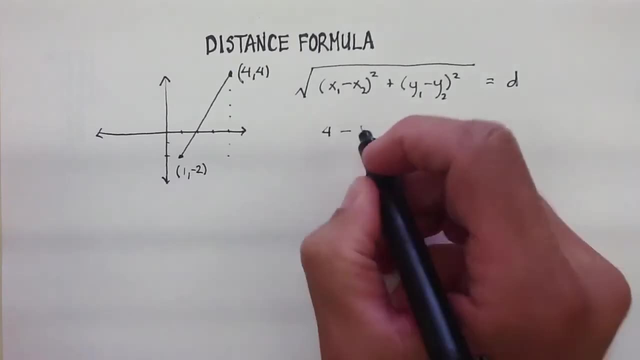 We'll just make this one the x1 and the y1, okay. So x sub 1 is 4, minus x sub 2, which is down here, which is 1, quantity squared: let's put this all under the radical. 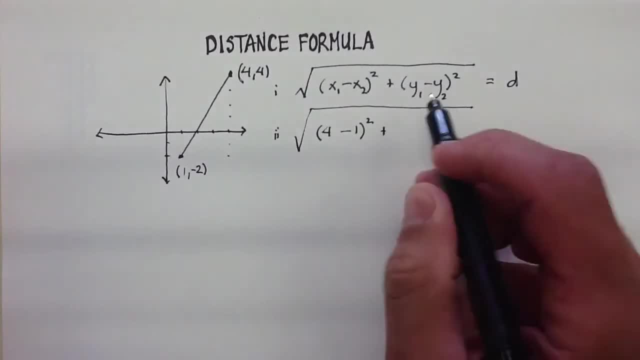 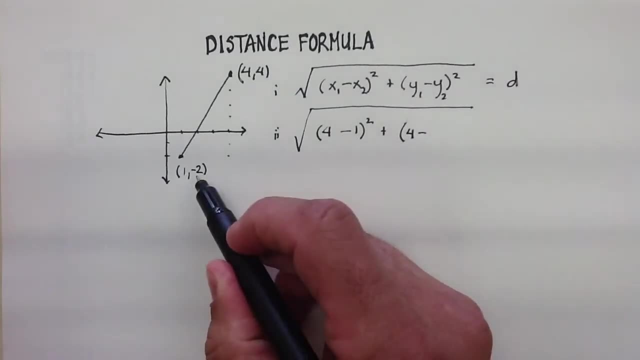 that's my first step, that's my second step, plus the difference between the two y's. so again, it's y sub 1,, which is 4,, minus y sub 2,, which is a negative 2,. all right, 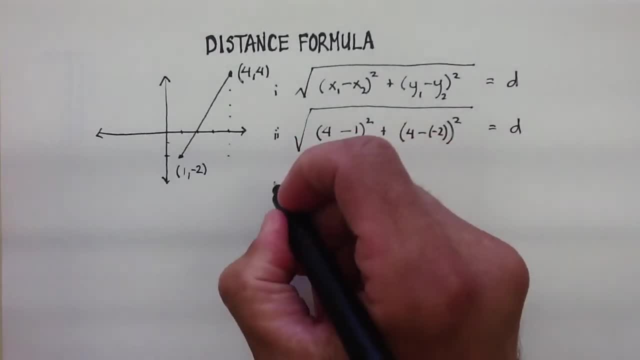 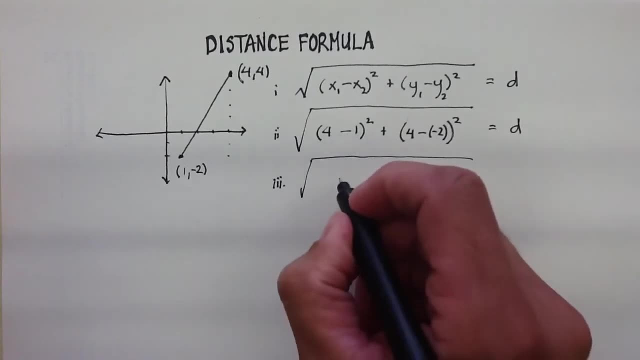 And then that should be equal to that distance. Let's go ahead and work this out. I'm going to get. the square root of 4 minus 1 is 3, squared plus 4 minus a negative 2, makes that a positive. 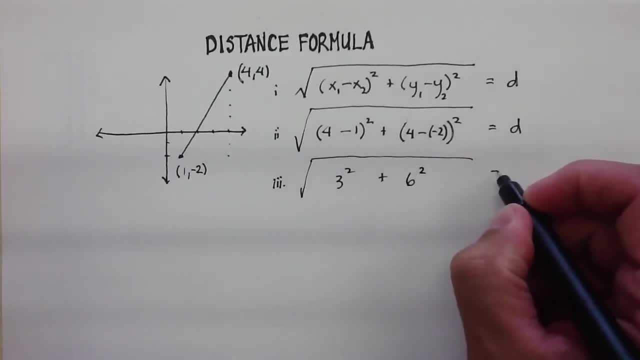 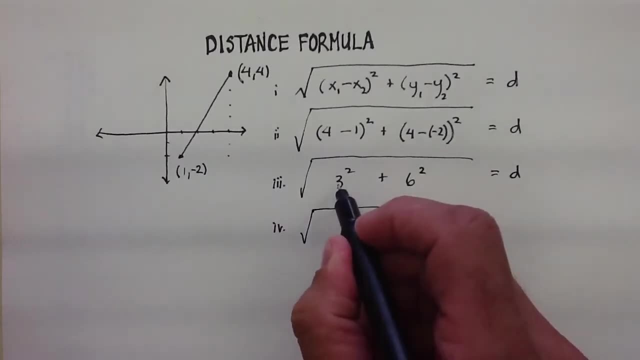 so that's going to be 6. quantity squared is equal to the distance. fourth step: that's going to be the square root of 9 plus 36, again, that's equal to my distance. and that's going to be last step. 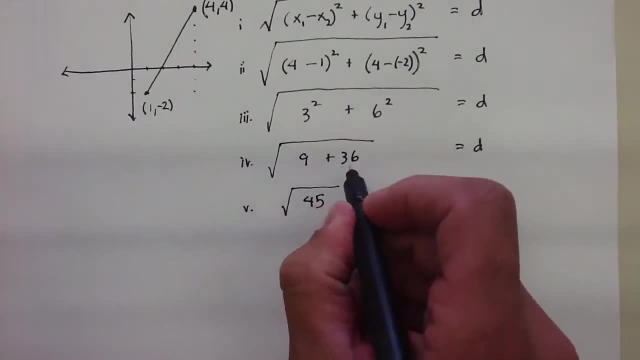 the square root of 45, because 9 plus 36, and if your teacher might ask you to go ahead and simplify this right, Either by estimating what the square root of 45 is or by writing it in a radical form, okay. 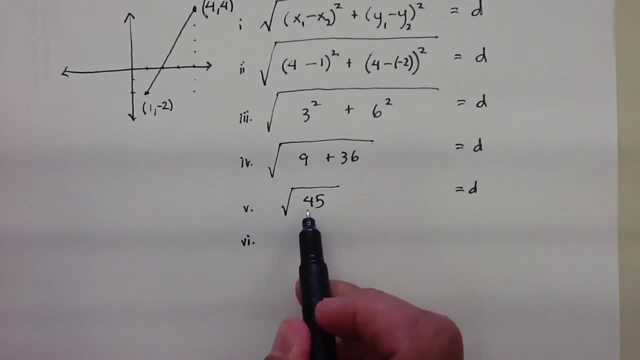 Now let's see if we can remember how we did it in radical form. One of the techniques is you take out the perfect square factors in here, so I can rewrite 45 as a square root of 9, times the square root of 5,. 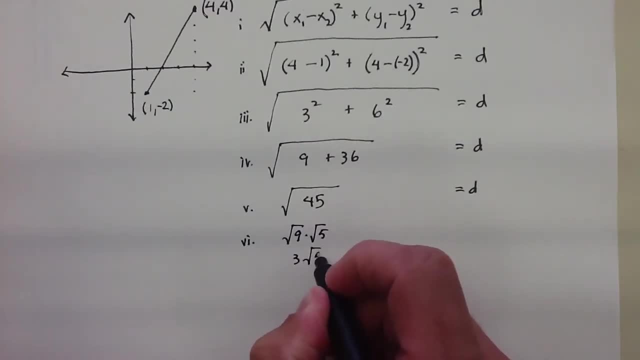 that's a perfect square, so you're going to get 3,. radical 5 would be that distance here. okay, And that's equal to the distance. The other way of doing this is you'd have to guesstimate what the square root of 5,. 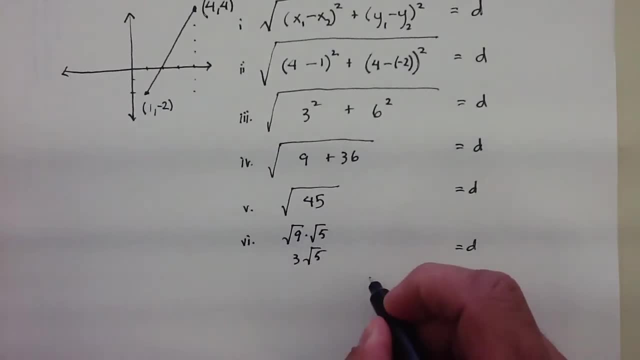 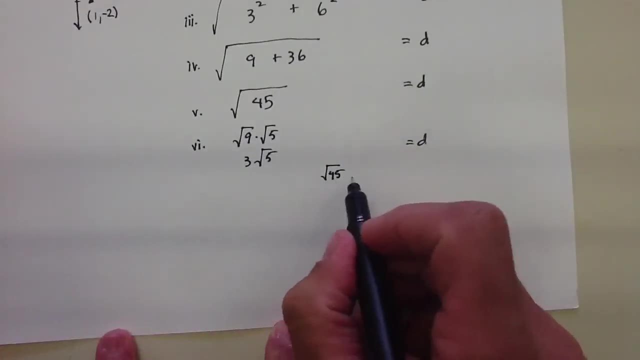 or actually what the square root of 45 is, and I'll show you a really cool technique. Here's 45, and what I do is I ask myself: what are the two perfect squares on either side of 45?? Well, I know that one perfect square is a square root of 36, right? 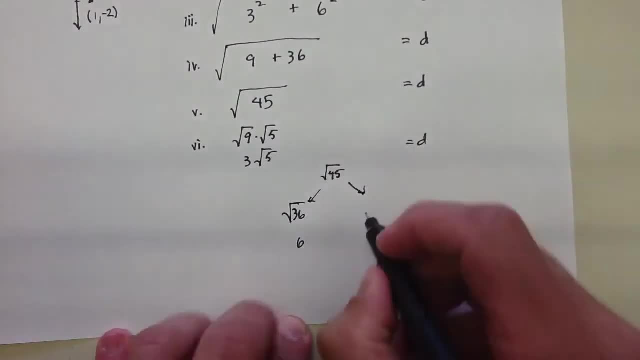 And that would just be 6.. I know, the other perfect square is a square root of 49,, right, And that's just 7.. So 45,, a square root of 45, is between the square root of 36,. 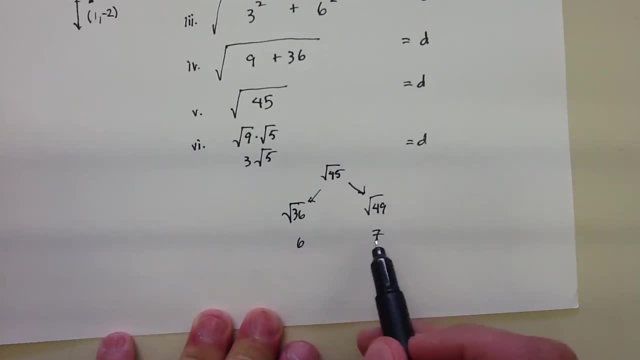 and the square root of 49, which means that it would be somewhere between 6 and 7.. And I'll show you how I show my students to guesstimate that. I say basically, the distance between 36 and 49 is 13.. 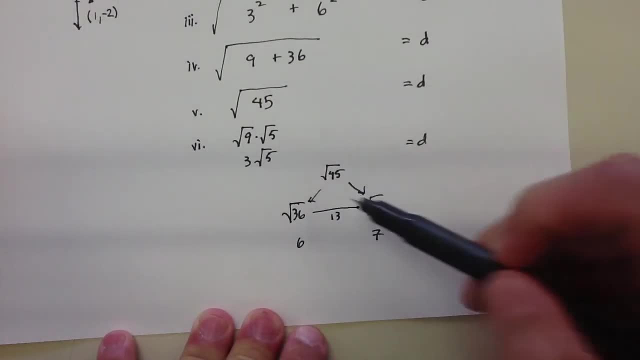 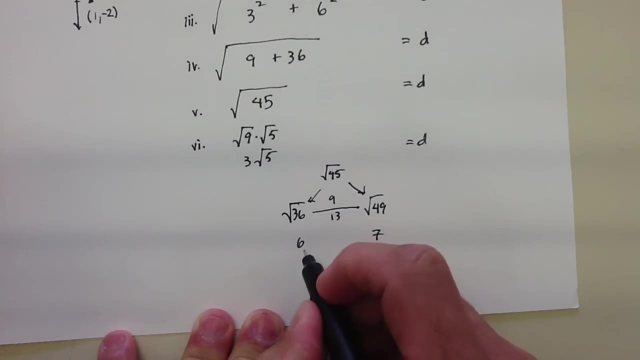 The distance between 36, and 45, is 9.. So the square root of 49 is basically 6 and 9 thirteenths. Okay, And that would be like an approximate answer. And if you go ahead and use your calculators, 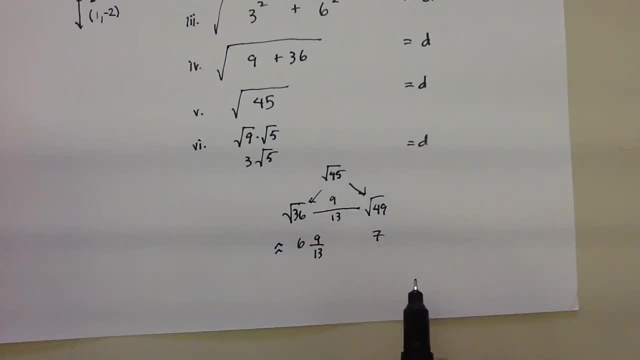 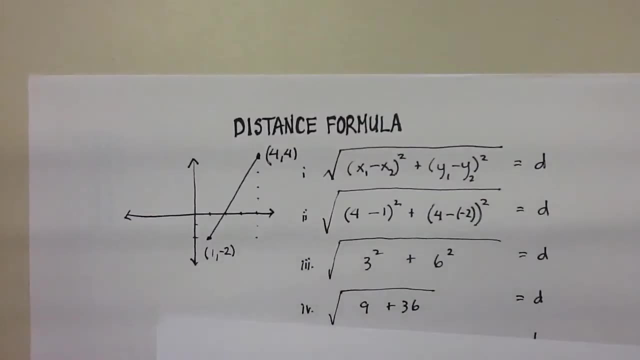 you'll see that's about right, And if you can reduce 9 thirteenths, that's fine in your own head. Now I want to show you something else with this distance formula. Okay, Let me just go ahead and recreate. 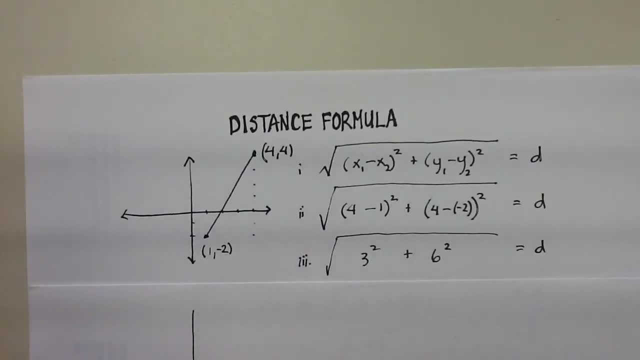 the exact same problem once again. So we had x and y axis, We had 1, negative 2.. So there is that one point: 1, negative 2.. We also had 4 and 4.. So 1,, 2,, 3,. 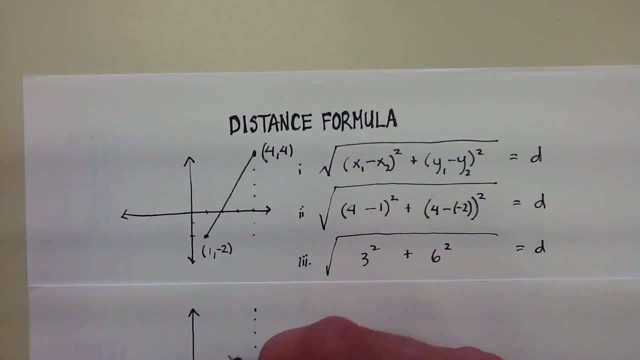 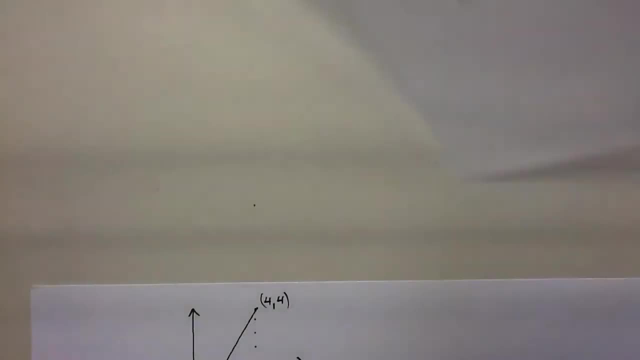 4.. 1,, 2,, 3,, 4.. So there is 4, 4.. We're trying to get that distance Okay, So let's go ahead and look at that. What if I forgot the distance formula? 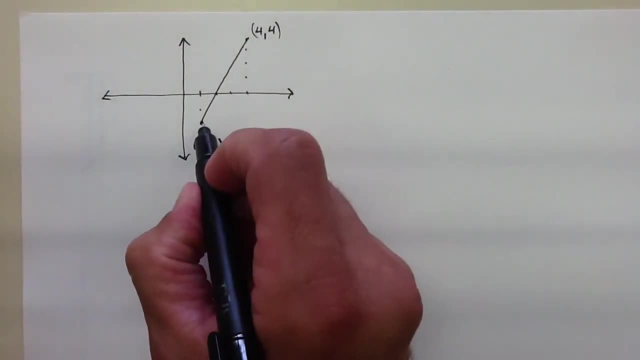 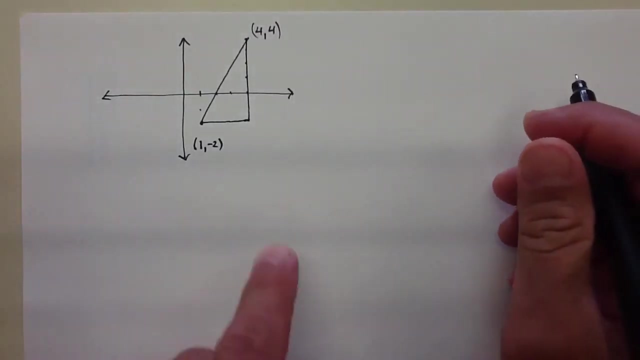 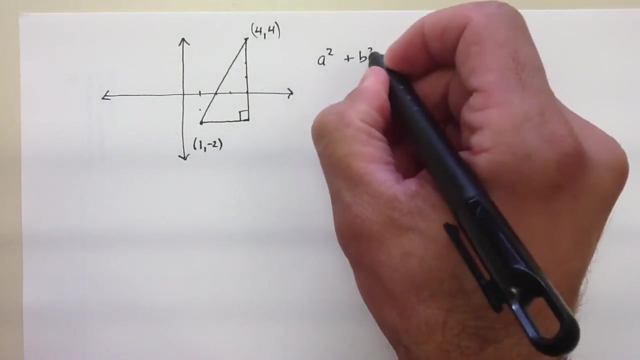 What if you just couldn't remember it? Well, I want to show you something. You can actually make this a right triangle. And if you can make it a right triangle, remember you can use the Pythagorean theorem, which is a squared plus b squared. 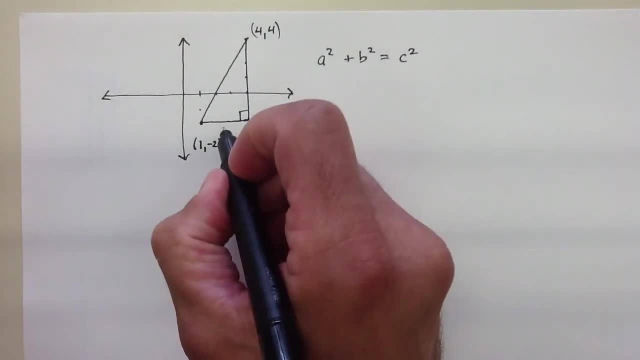 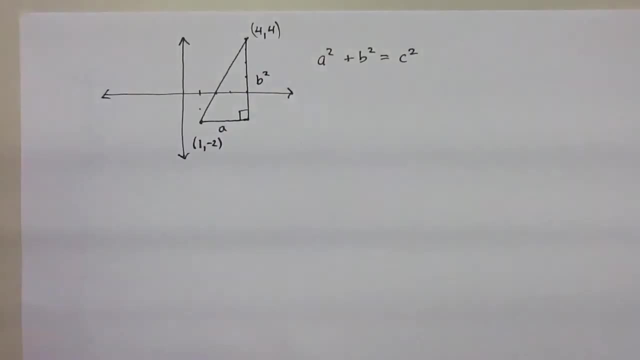 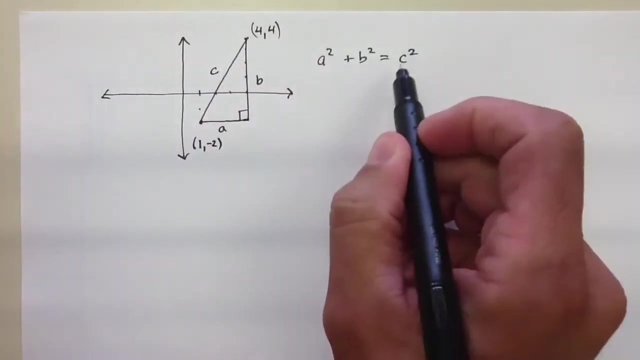 is equal to c squared. In other words, this side squared plus this side squared- Oops, shouldn't have put the square there. That side plus that side right would be equal to that side squared, Which is really the hypotenuse.